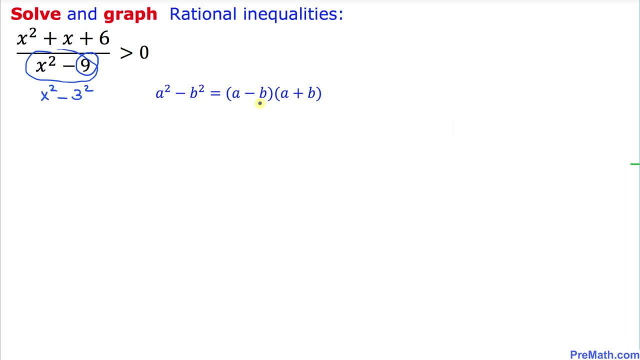 a squared minus b. squared is always equal to a minus b, b times a plus b, So this could be written as x minus 3 times x plus 3.. So far, so good. Now let's focus on the numerator x squared plus x plus 6.. And we have copied it down right up here: 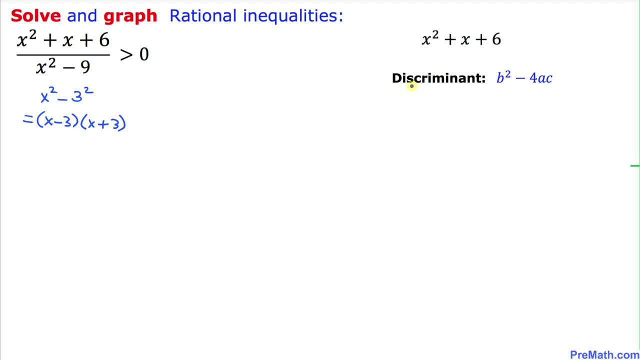 on the right hand side. Now we are going to calculate the discriminant of this quadratic expression: x squared plus x plus 6.. And always remember that discriminant is equal to b squared minus 4ac. So this, in our case, a is going to be equal to 1,, b is 1, and c is 6.. 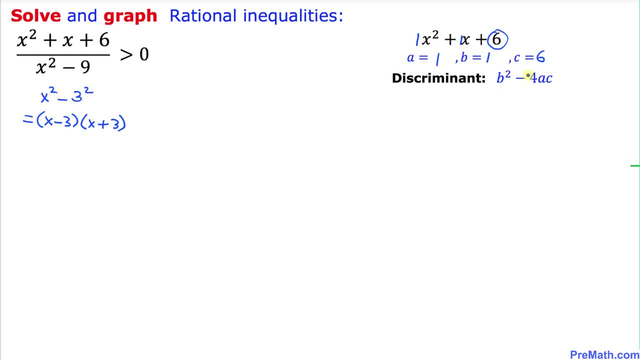 So let's substitute these a, b, c values in this: b squared minus 4ac. That is going to give us 1 squared minus 4 times 1 times c is 6.. That is going to give us 1 minus 24.. That is going to give us: 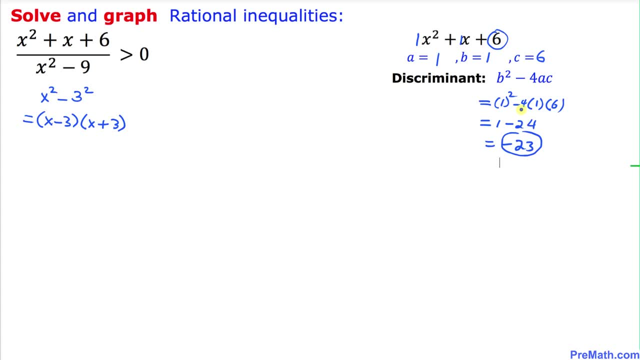 negative 23.. So thus our discriminant turns out to be negative 23.. And one more thing just keep in your mind: a quadratic is factable if its discriminant is either 0 or a positive Perfect square. And since this discriminant is negative 23,, therefore, this numerator is not. 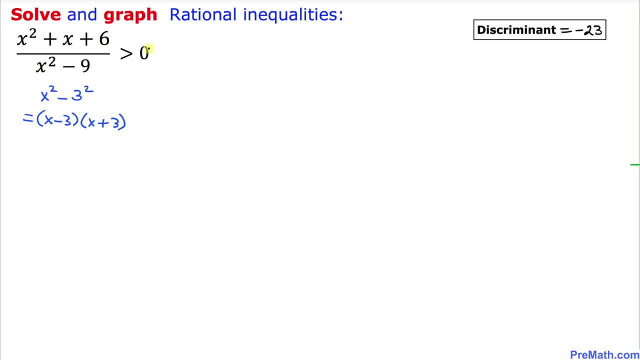 factable. So thus we can write this inequality as nicely. we can write as: x squared plus x plus 6 on the top is not factable. We're going to just just leave it alone. And the denominator is: could be factored to x minus three times x plus three, which is greater than zero. And here I have wrote down in a: 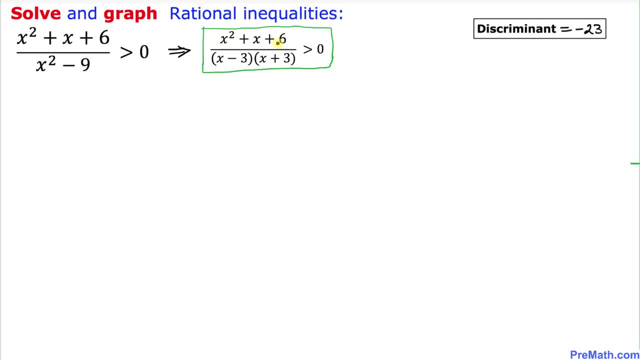 neat way, And I am going to call this, inequality is and I I stands for inequality. And now, in our next step of we are going to find the critical values, to find the critical values, we are going to numerator and denominator, both of them equal to zero, just the numerator and these denominator. 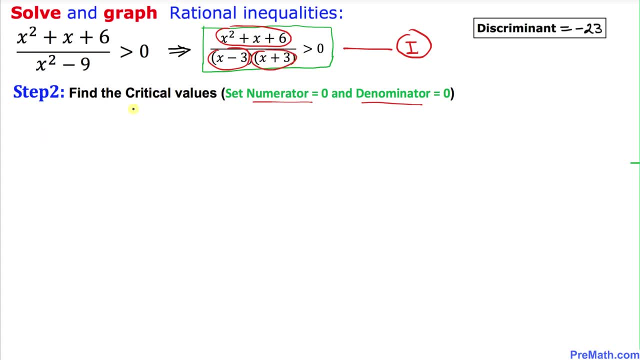 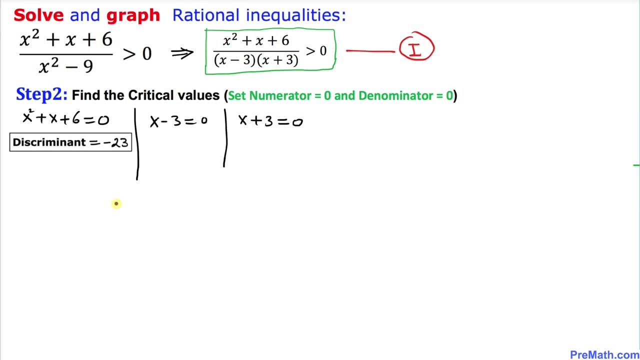 all of these one. so let's go ahead and do that one. the numerator is x square plus x plus six, let's set it equal to zero, and the denominator is x minus three, equal to zero. and the other one denominator is x plus three, equal to zero. and for this quadratic part we just calculated. 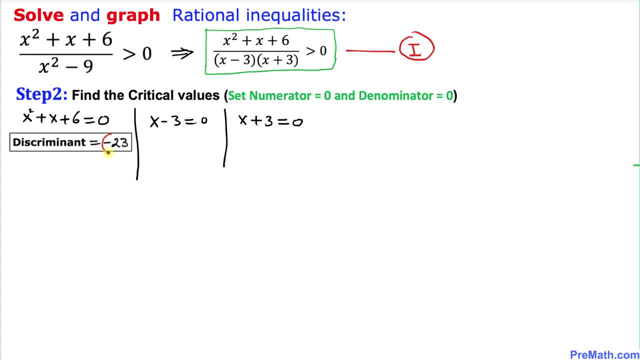 discriminant turns out to be negative. 23 in our previous step and by looking at this, chart over here our discriminant, since it is negative. so this tells us that we have no real solutions. so therefore it has no real solutions. no real solutions now. let's move on to x minus three, equal to zero. that is going to give us. 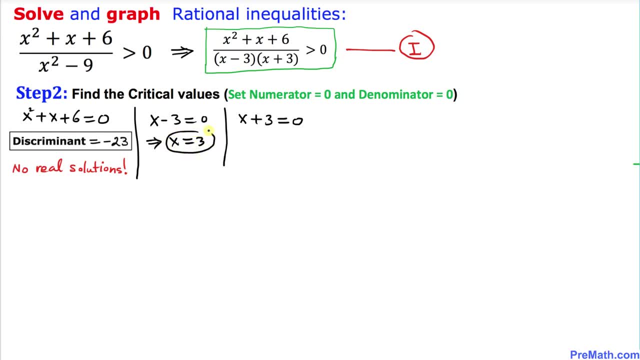 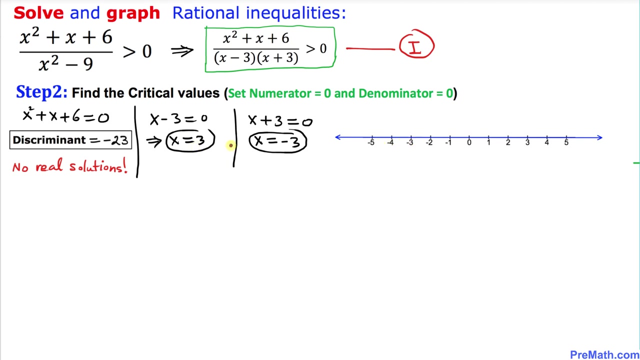 x equal to positive three, and here this is going to give us x equal to negative three. so thus we got two critical points: x equal to three and x equal to negative three. and here is is our real number line and we are going to locate these critical points. so the first one is x equal to 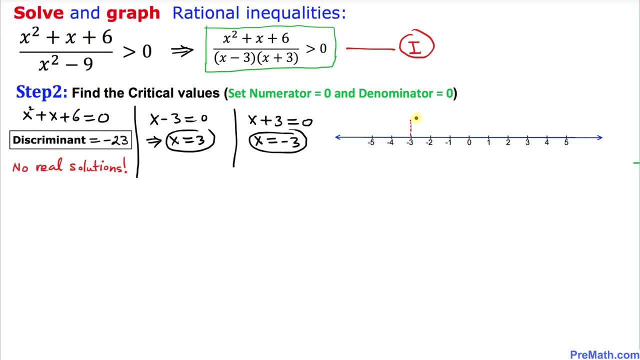 negative three, i am just going to put this kind of dotted line on the top. and for x equal to positive three, i'm going to put a dotted line as well. now let's put this x equal to three value. in this inequality i- and here is our inequality i. let's go ahead and 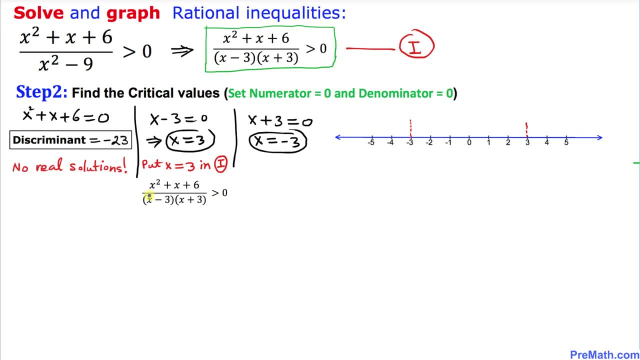 replace x equal to three value. let's look at at the denominator: this is x. if i replace this x by three minus three, that is going to give us zero, and we know that whenever we have a zero at the denominator, this will be undefined. just keep in your mind. so, therefore, at this point, x equal to 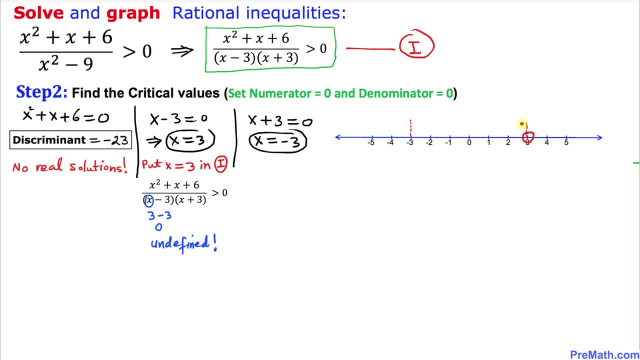 three. we are going to have an open circle. so this is the zero and we are going to have an open circle circle. now we are going to repeat the same process for x equal to negative 3. so this is what i wrote down. put x equal to negative 3 in this inequality i. this is right up here. once again, look at the. 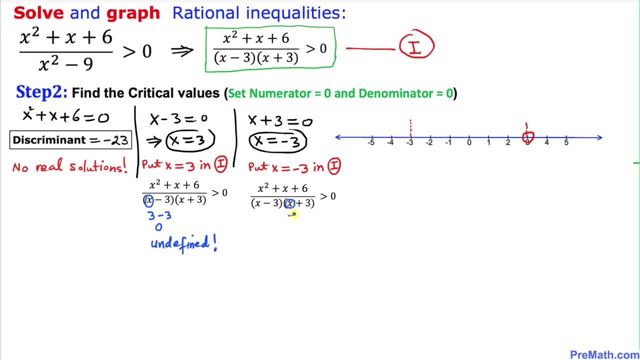 denominator. if i replace x by negative 3 and this positive 3, that is going to give us a 0 whenever we have a 0 at the denominator. this is going to become undefined as well. so therefore we are going to put a open circle on negative 3 as well. and one more thing: these two critical 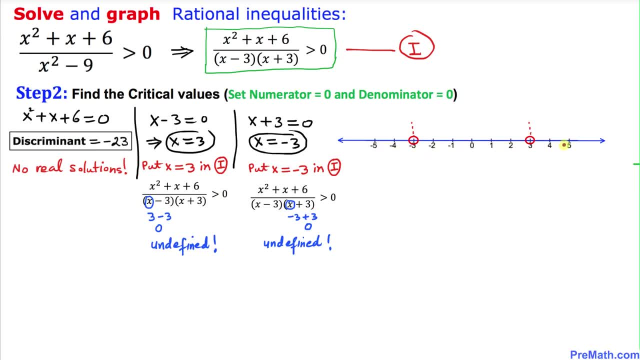 values divide this real number line into three regions, three parts. the first one is on the left hand side of this, negative 3. so i'm going to call this region a and this region between negative 3 and positive 3, i am going to call region b, and the region on the right hand side of this point 3, i am going to call 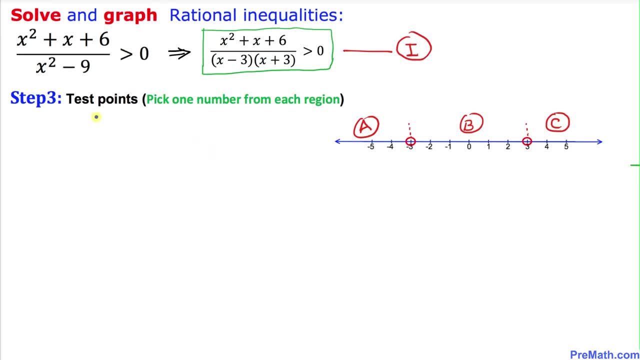 region c. and here is our next step. we are going to test points. in other words, we are going to pick one number from each region, and now let's focus on region a. here i am going to pick one point. let's pick x equal to negative 4. that looks a reasonable point, and now we are going to put this x equal to. 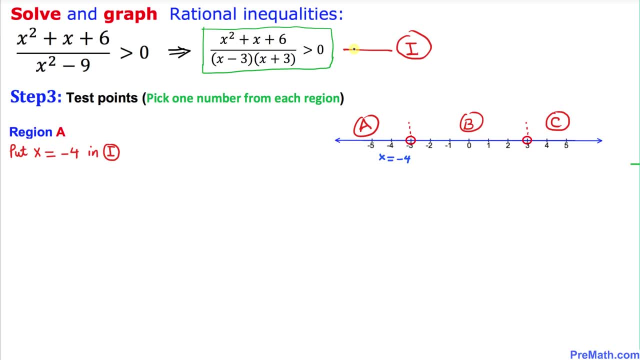 negative 4 value in this inequality i, and here is our inequality i. and let's go ahead and replace x equal to negative, And this is going to become negative 4 squared plus negative, 4 plus 6 divided by negative, 4 minus 3 times negative, 4 plus 3.. 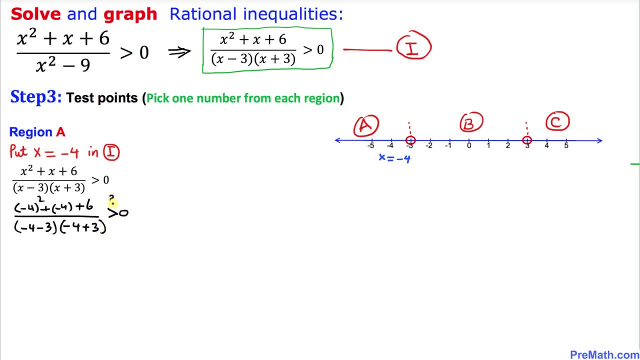 And we're going to check whether this statement is true or false. And now let's simplify the numerator. That is going to become 16 minus 4 plus 6, divided by negative, 7 times negative, 1 greater than 0.. As we can see that our numerator is going to have a positive number, We are just interested in the sign, not the number. 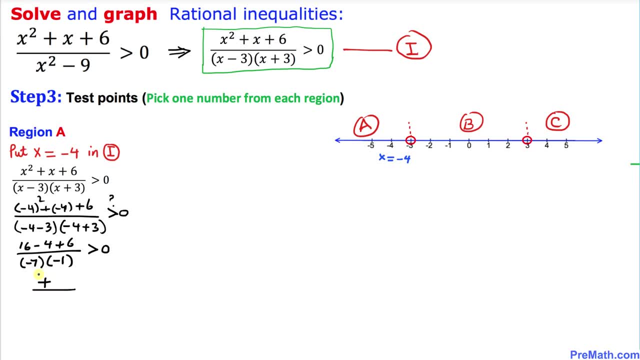 So it's going to be a positive sign and divided by this, negative And negative become positive sign as well. It is greater than 0 and positive divided by positive is positive, is greater than 0. That means this statement is indeed true. So therefore, this region A- I am going to put true for this region A- 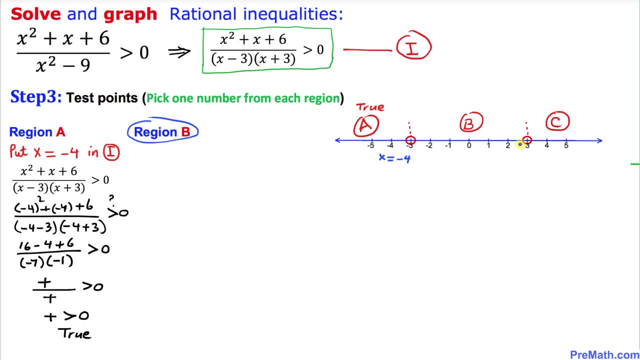 Now let's focus on region B and we are going to pick one point, And this time I'm going to pick x equal to 0. And now we are going to put x equal to 0 value in this inequality I which is right here? 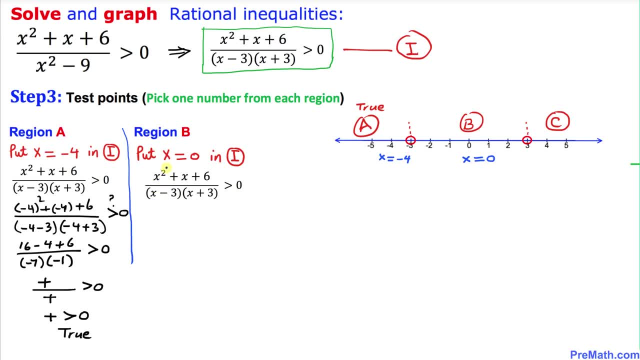 Let's go ahead and fill in the blank. Wherever we see x, we are going to replace it by 0.. So this is going to become 0 squared plus 0 plus 6 on the top divided by 0 minus 3 times 0.. 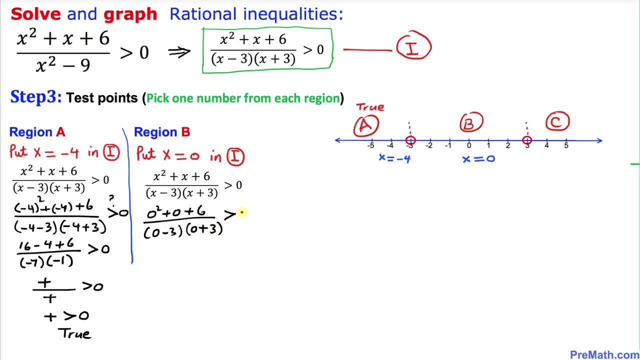 Plus 3 is greater than 0.. Let's simplify: at the top That's going to become positive 6 divided by we got negative 3 times positive. 3 is greater than 0.. As we can see on the top, our sign is positive and the denominator negative 3 times 3 is going to become negative 9.. 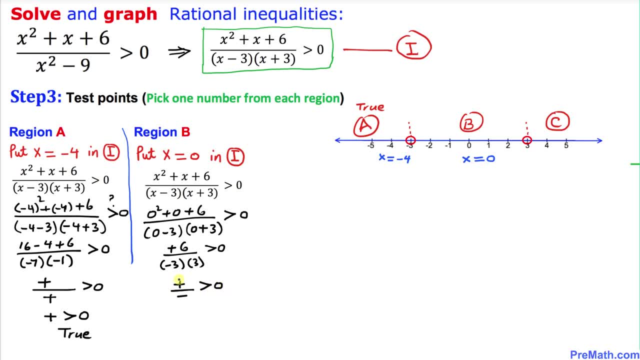 So it's a negative sign. So, once again, positive divided by negative is going to give us negative is greater than 0. And we can see that this is statement is false. So therefore, our region B is going to be false. And now let's focus on region C. 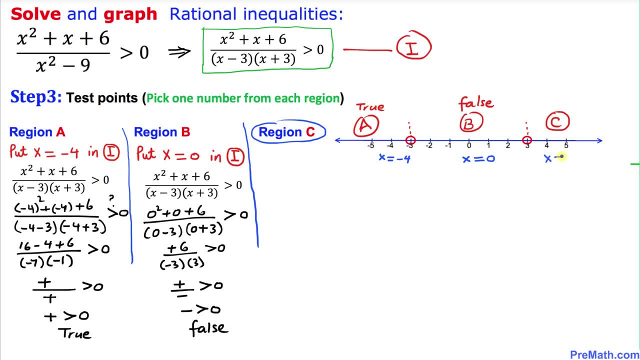 And in this region I am going to pick x equal to 4 point And let's put x equal to 4 value in this. So let's go ahead and replace x by 4.. So this is going to become 4 squared plus 4 plus 6. divided by 4 minus 3 times 4 plus 3 is greater than 0 on the top. 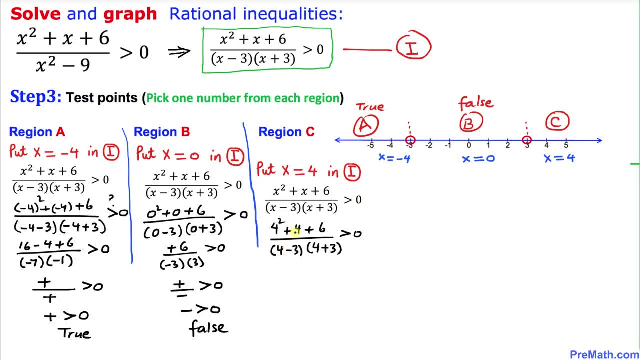 That is going to give us: 16 plus 4 is 20.. And 20 plus 2 is going to give us 0.. That is going to give us 26. divided by that is going to give us 1 times 7, which is greater than 0. 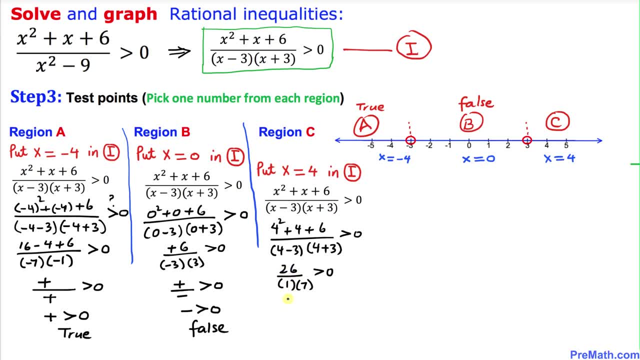 So we got this is the top sign is going to be. numerator has a positive sign and the denominator has a positive sign as well. So that is going to give us positive is greater than 0, which is a true statement. So that's it. 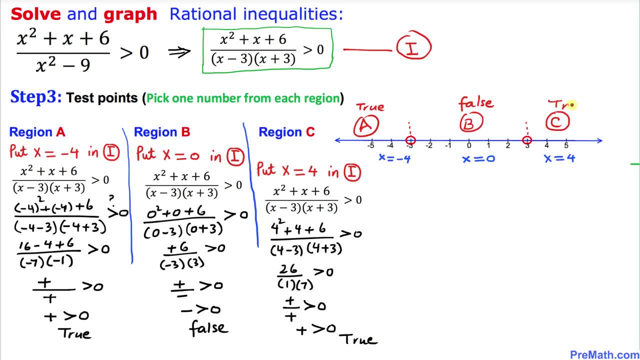 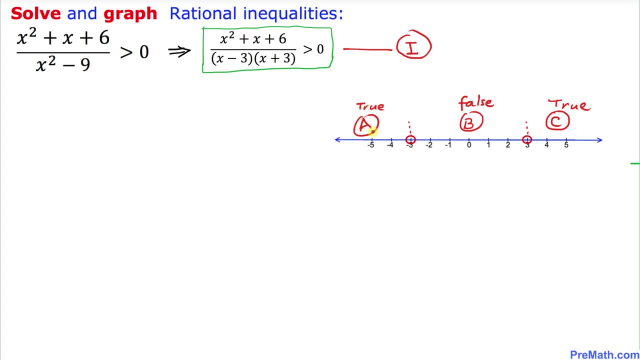 Thus, our region C is going to be true. And here is our final step: Let's go ahead and shade the region. whichever is true, A region is true, So I am going to shade this part. region A- All right, And region B is false. 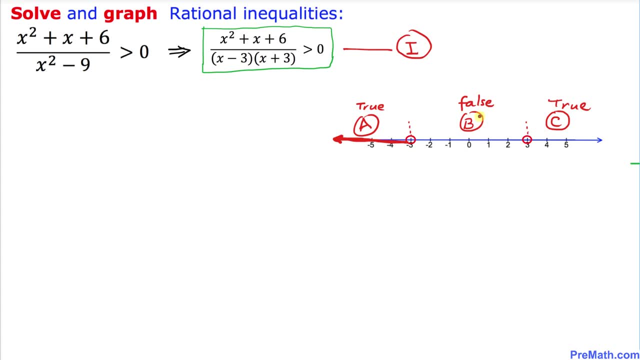 We're going to just simply ignore it. OK, so we're going to rule this one out And let's look at region C, which is true as well. So I am going to shade that region as well, And just over here, since this is going on the left hand side, so left hand side means that's going to be negative infinity.